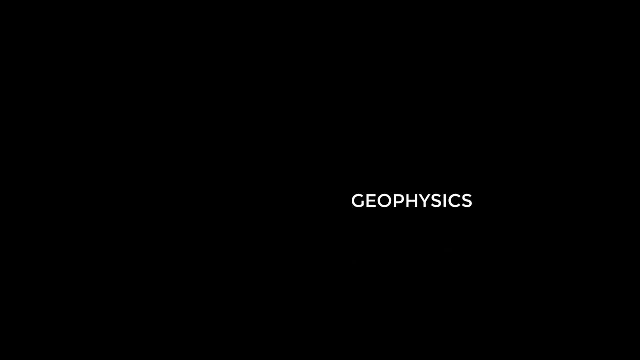 study geophysics, one of the major branches of geoscience that applies the principles of physics to the study of the Earth. Geophysicists connect the physical processes that we see and experience on the surface of the Earth, like earthquakes and volcanoes, to processes 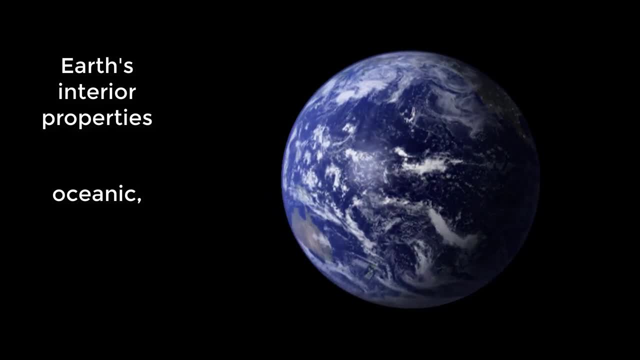 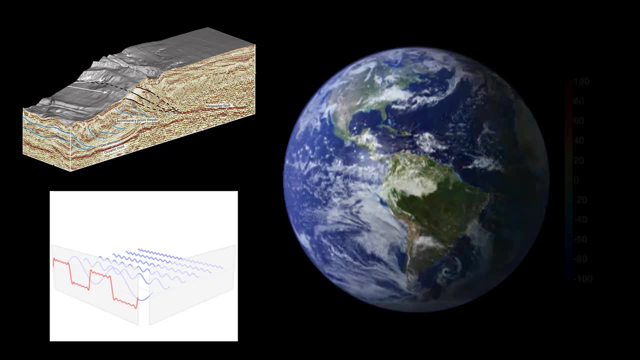 driven by the Earth's interior properties or affected by oceanic, atmospheric and solar forces. Geophysicists examine what's inside the Earth at large and small scales, conducting surveys and generating maps of Earth's physical fields, often without disturbing the surface. 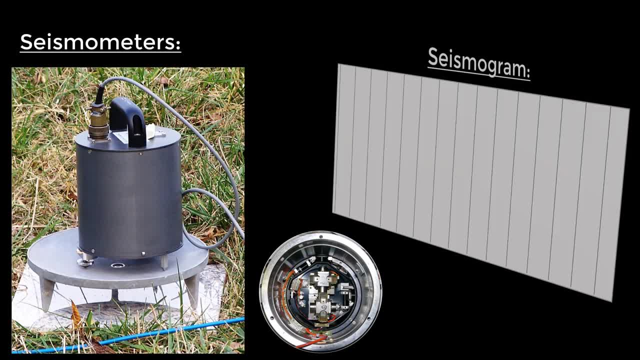 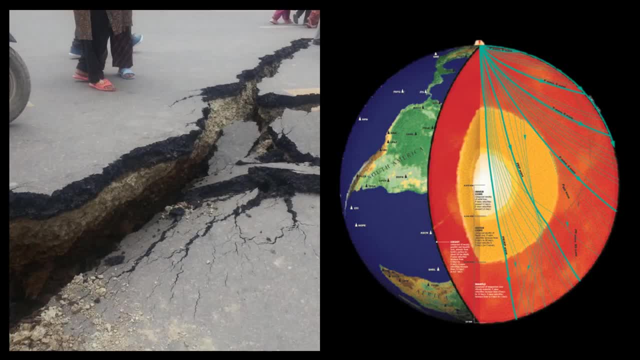 What does that mean? Some geophysicists install instruments called seismometers to study earthquakes' impacts on people, as well as what earthquakes can reveal about Earth's internal structure and composition. They can create numerical models to measure and forecast how the ground 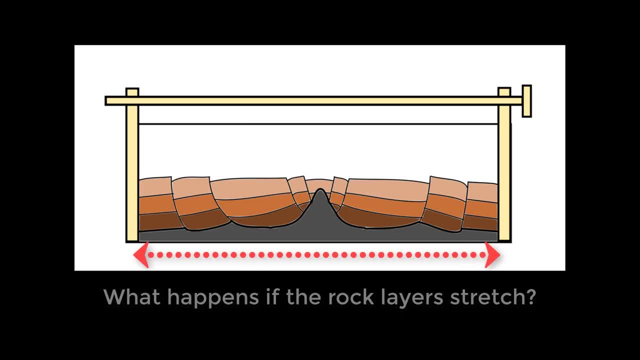 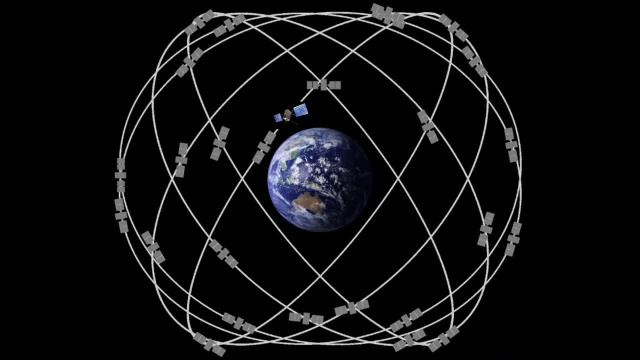 might behave in a future earthquake. Some geophysicists use satellites to understand the Earth's changing shape and gravity field, such as the Global Navigation Satellite Systems, including the Global Positioning System or GPS, which people use to navigate Many geophysicists. 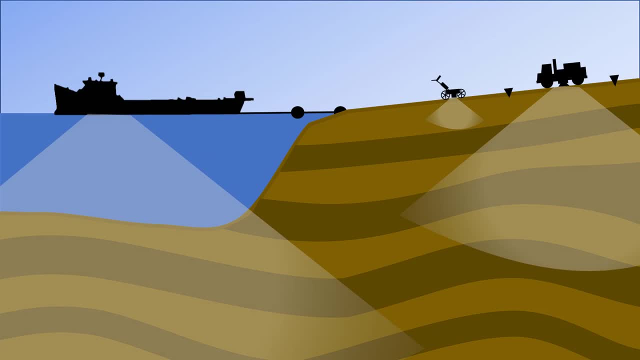 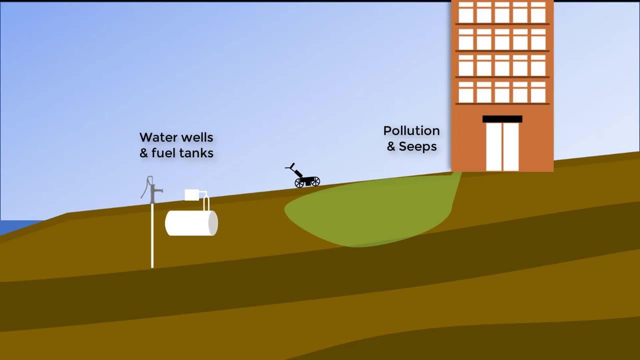 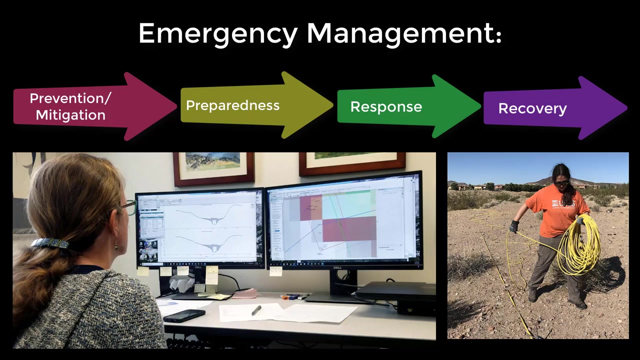 use probes carried by ships, boats or land rovers to scan for useful resources such as groundwater, metals and hydrocarbons. Others use them to evaluate human impacts on water quality or to work with emergency management teams for mitigation and planning around natural hazards such as tsunamis, volcanoes and landfills. 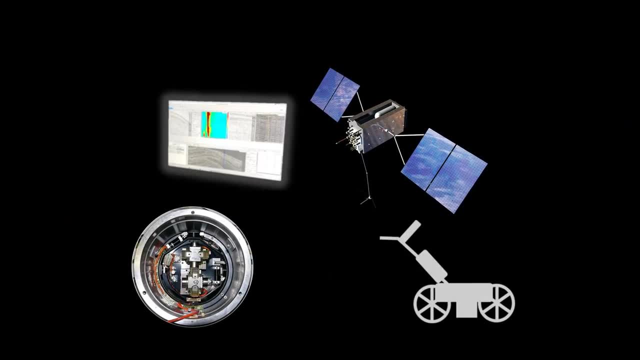 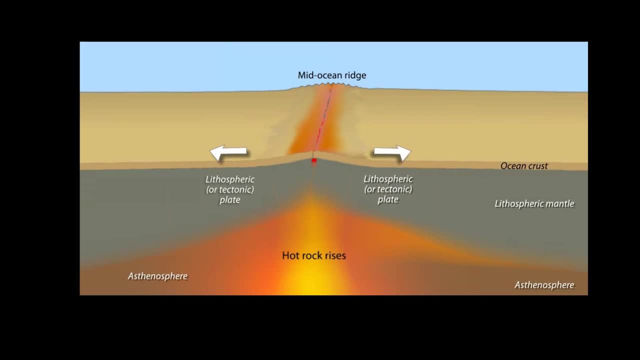 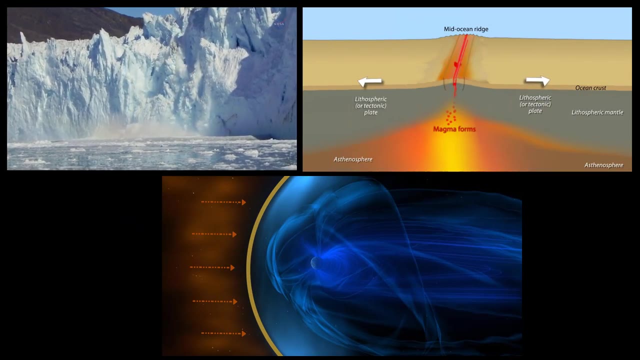 Some geophysicists use a combination of these tools and techniques to focus on big-picture ideas in science, like visualizing and explaining how plate tectonics functions, how our magnetic field protects us from the sun, or how climate change has and may continue to affect our 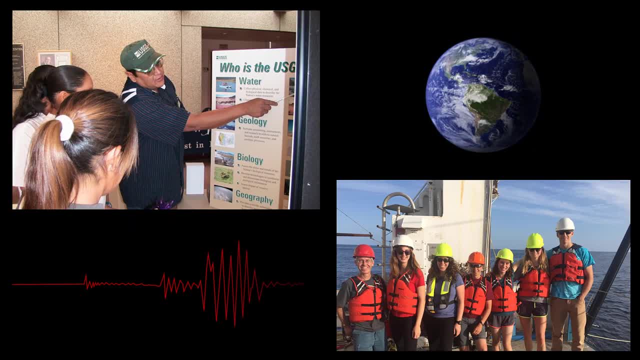 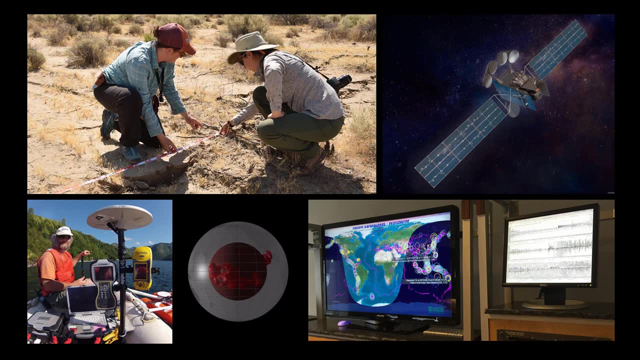 planet Together. all of this work shows how geophysics is a dynamic, innovative field that seeks to answer many of the most fundamental questions about our planet and how we can live on it safely. For more information, visit wwwgeophysicscom.